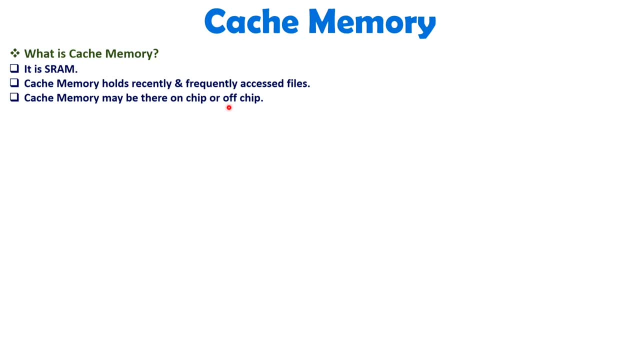 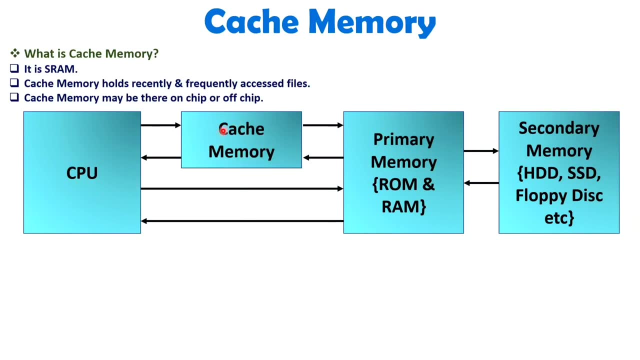 explain you how it is organized with computer system. so here you see, we have cpu and nearest to the cpu we have cache memory. so data mapped with cache memory directly accessed by cpu. so with cache memory there will be recently and frequently accessed file. that's why access of 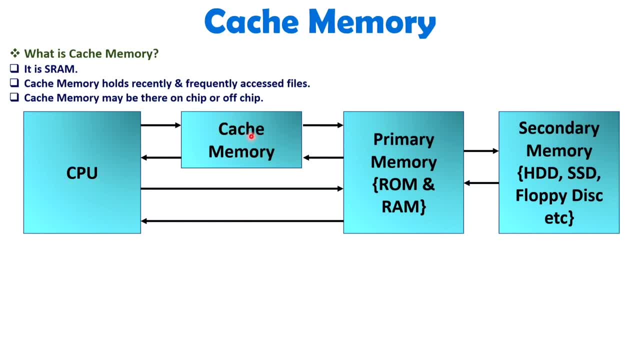 data. that will be very fast with cpu, along with cache memory. cache memory will map data inside primary memory, and primary memory will map data inside secondary memory. primary memory may be ram and rom and secondary memory that may be hard disk or it may be ssd or it may be floppy disk. 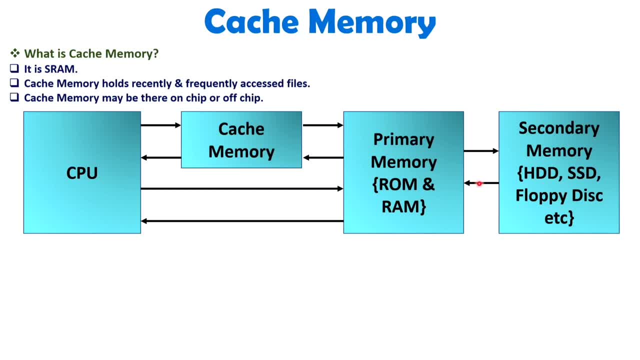 here. my dear students, you should understand one thing here: access of data with cpu will happen with cache memory in majority of cases. that's why it will holds recently and frequently accessed file and management of this cache memory. that will happen with respect to operating system inside cpu. 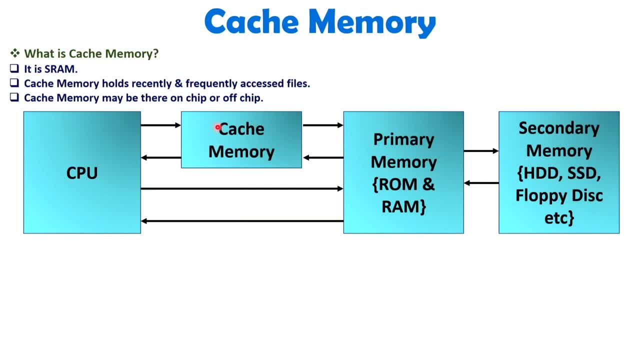 so operating system will give commands to cache memory based on what file should be loaded over here, and those files will be majority of times based on recently and frequently accessed file. so accessing of data with cpu will be very fast and that mapping will happen with respect to primary and secondary. 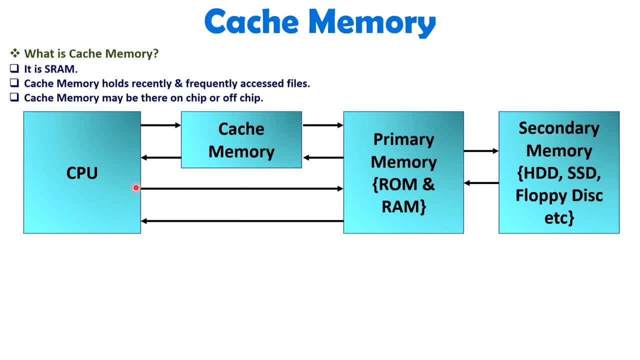 memory. let us discuss first few basics which is there with cache memory. so you should know, my dear students, cache memory is small in size and it has fast data access. how fast data access is there? that even i'll explain you when i explain levels of cache memory right now. just consider it will. 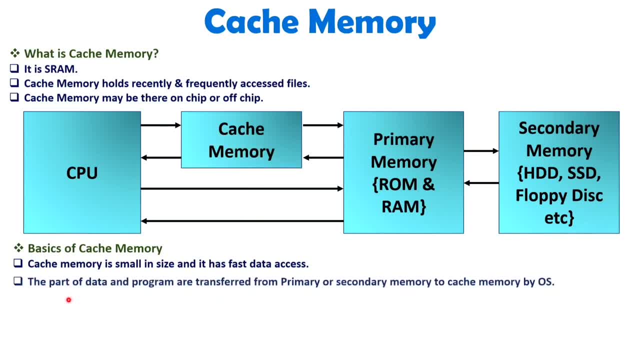 be having faster operation here. you can see that, my dear students, when we talk about execution of program or data, then first of all that program or data that will get transferred inside cache memory from primary or secondary memory, and here that will be done by operating system, right? so operating system will decide that which files that should be. 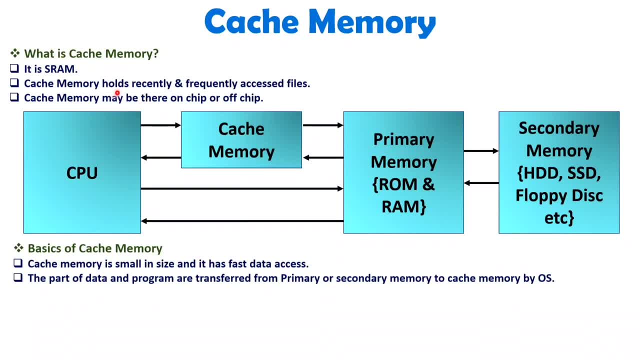 there in cache memory and that should be recently or frequently accessed file in majority of cases. normally we would write code here or showed code, say this kind of cpu of cache error, what you made. if a cpu is in original state, then this is notmay be wrong. if pedal gathered set is, shall also be. 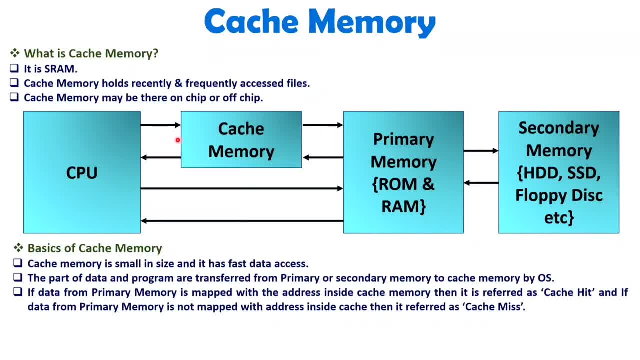 here, my dear students, you will be observing that primary memory is mapped with cache memory and whatever cpu is asking for data and as if it is available with cache memory, then that is referred as cache hit. but as if the data asked by cpu is not available with cache memory, then you can say: 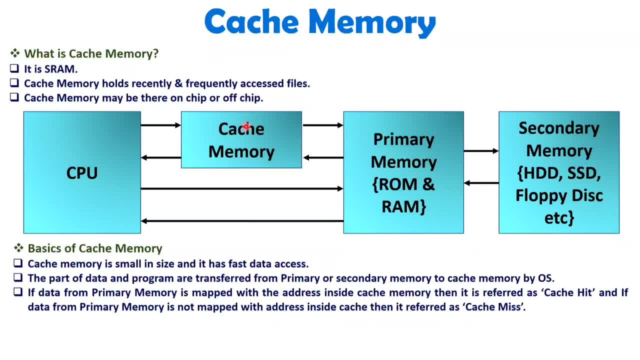 will map that data inside primary memory, It will take it over here inside cache and then access will be given to CPU. Here, my dear students, if data is not available, then by different mapping techniques. cache memory will take data from primary or secondary memories. 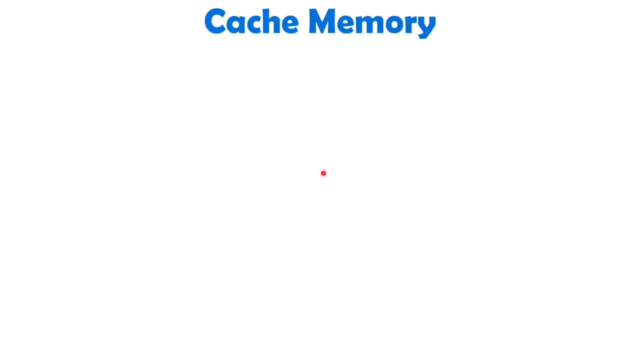 Now, my dear students, I'll be going to explain you different levels of cache memory. So here let us try to understand. first level one cache memory. And, for example, here I have considered advanced microprocessor in which we have multiple core. So here we have one system of microcontroller. 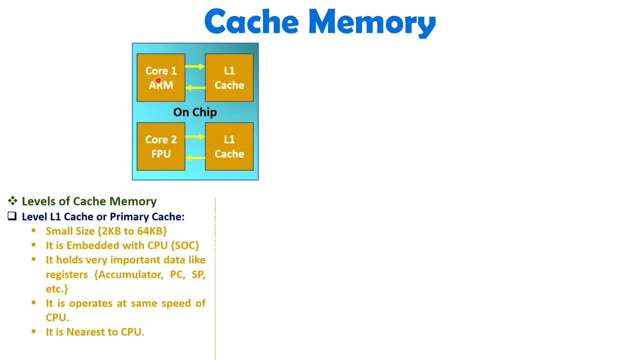 in which we have two cores. One core is there with ARM, Second core is there with floating point unit. And then you see, here on chip we have L1 cache memory, So you should know microprocessor. So here we have L1 cache memory, So you should know microprocessor. So here, 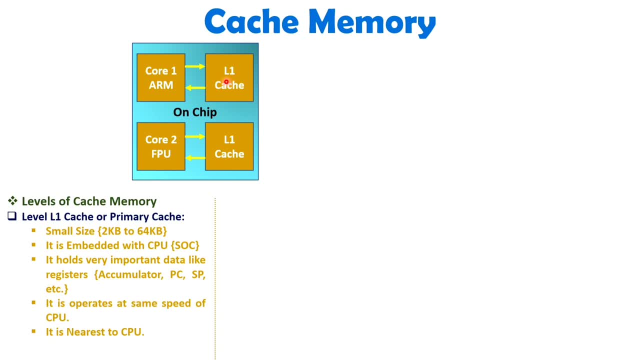 my dear students, L1 cache memory, that will be very small in size and it will be embedded on chip in majority of cases. right And here you'll be observing that it will be there with small size and that size is ranging from two kilo by two, four KB. Here, my dear students, you should know. 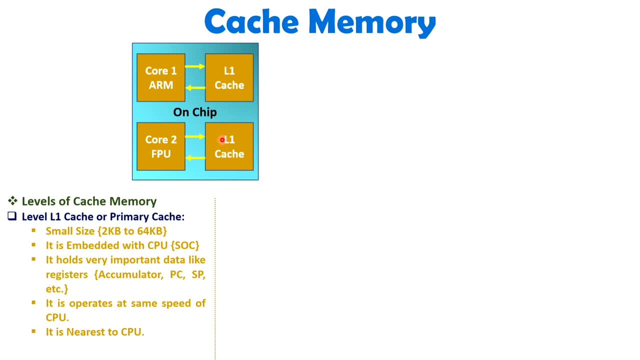 this L1 that is holding very important data, like it may be holding resistors, like accumulators, program counter, stack pointers, as well, as it will be having paging system enabled inside and which is having data related translation look aside buffer. So, based on L1, cache access will be: 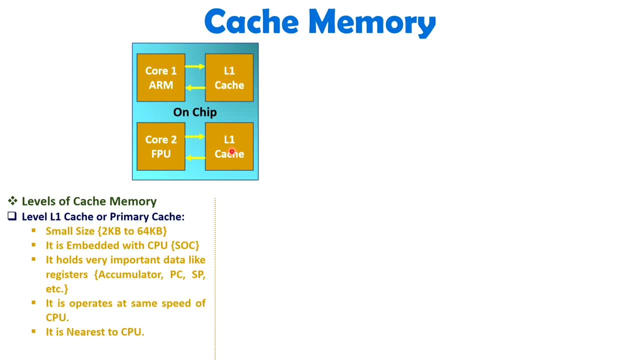 very fast Why? The reason is operating speed of this L1 cache memory. that will be same as CPU operating speed, right, And it is very nearest to CPU that you can see. After that you should have to see L2 cache memory. So L2 cache memory that is available over here and that is mapped. 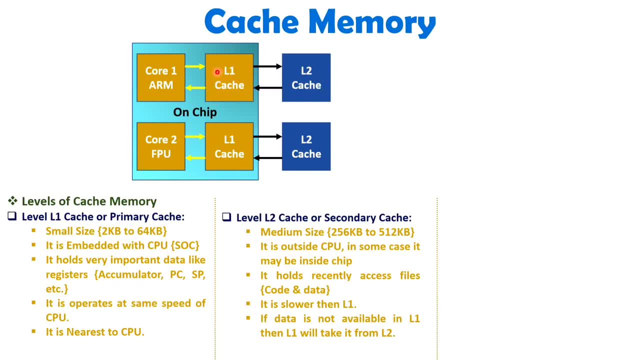 with respect to L1 cache. If you observe, here we have multiple L1 cache, So multiple L1 cache are mapped with L2 cache Here. size of L2: that is bit more compared to L1. It is there with medium size. It will be ranging from 256 kilobyte to 512 kilobyte. So this is the size of L2 cache. 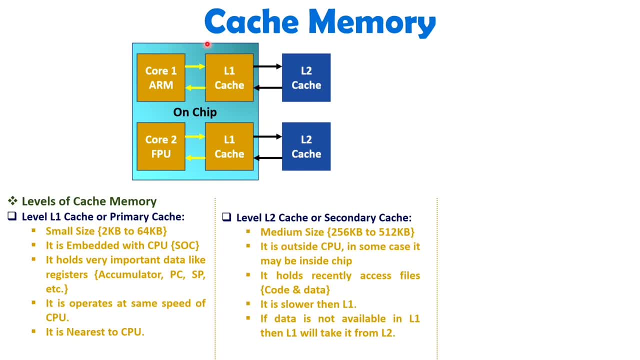 memory. It will be outside CPU. You can observe here we have chip that is CPU and this is outside CPU, right, It is holding recently accessed files. Those files may be code or data. It will be obviously slower than L1, right, And it will be mapping data from other memories, right Here. 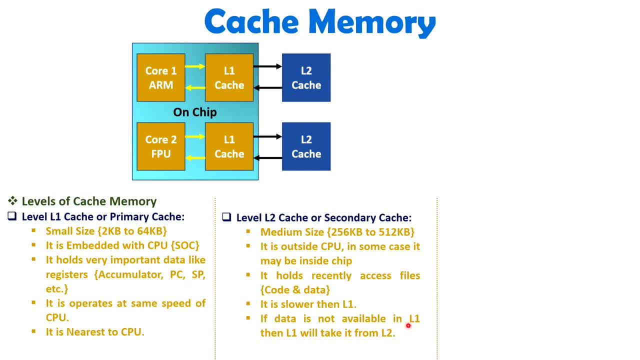 my dear students, if L1 is not available, in that case this core can directly take data from L2 cache, right? So L1 is not like it is always available. In few chips it may be there. If it is not there, then core can be directly interfaced with L2.. But you should. 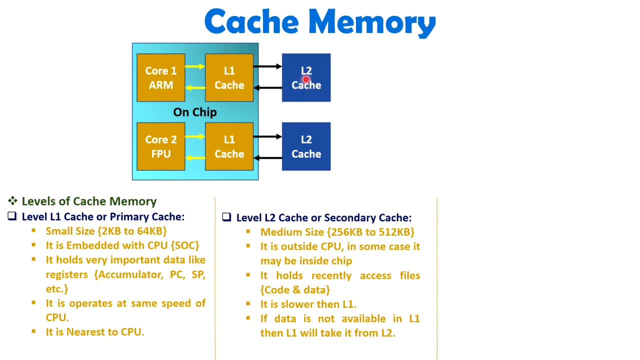 know L1 is on-chip cache memory and L2 is off-chip cache memory. After L2, you will be having L3 cache Here. my dear students, if you observe this L3 cache, that is common for L1,. 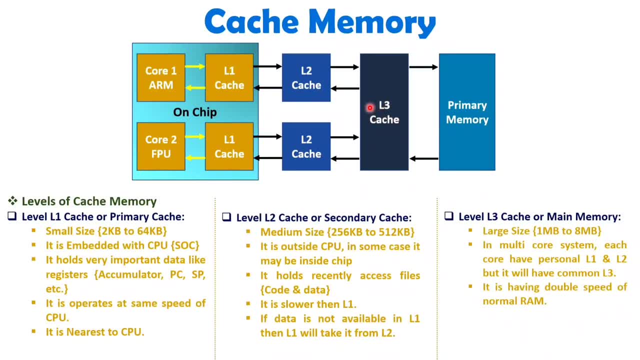 and L2, you see. So L3, that will be large in size compared to L1 and L2.. Obviously, it is far from this core compared to L1 and L2.. L1 is nearest. After that, L2 will be there And L3, that is. 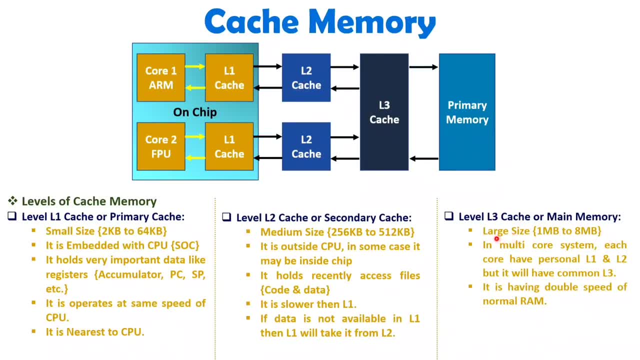 bit far compared to this too. Here you should know size of this L3. that is ranging from 1 MB to 8 MBs. Here in multi-core system you will be observing you may be having personal L1, and L2 for separate cores, But L3 cache that will be common for all the cores, right And here. 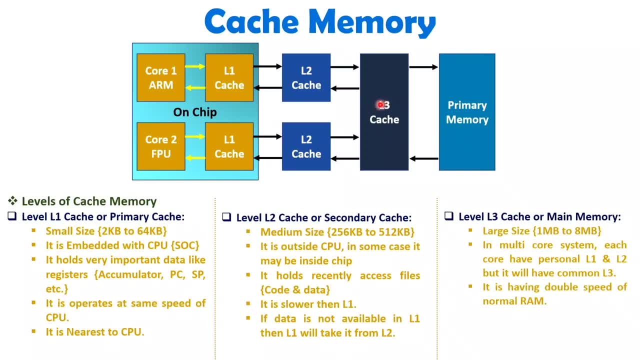 my dear students, you should know L3 cache that is slower than L1 and L2. But again it is having double of the speed compared to normal RAM. So here with primary memory, you will be having RAM and this L3 will map data from the RAM And compared to RAM available over here with primary 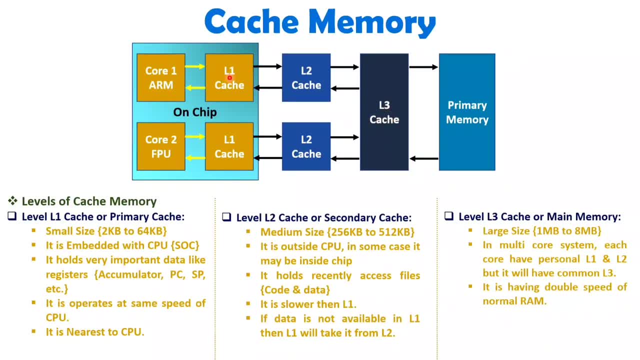 memory speed of L3, that will be doubled right. So that is how complete cache organization will be there in terms of L1, L2, and L3.. Nowadays in computer system with core i3, core i5,, core i7,. 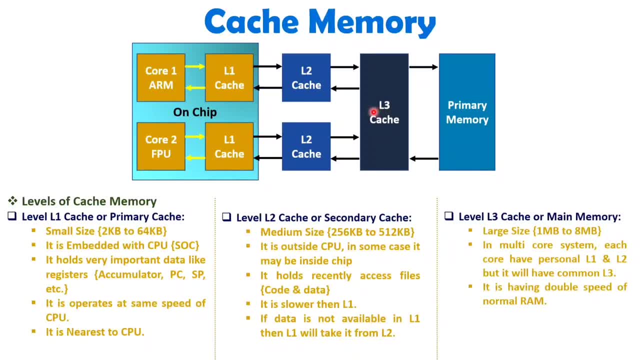 with 11th generation, we are having L4 cache as well, So that will be connected after L3, that is also off-chip. Remember this Now, my dear students, few important terminologies that I would like to discuss with you, like what is flush of: 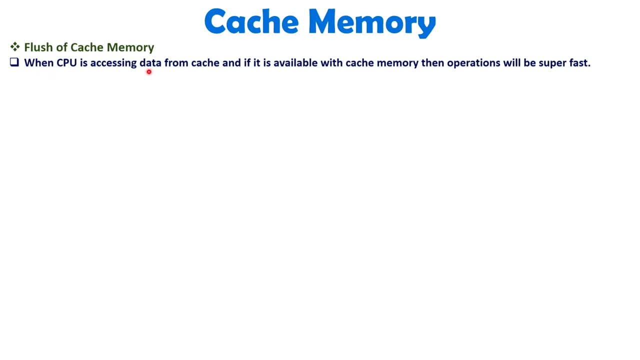 of cache memory. So you should know, my dear students, when CPU is accessing data from cache, if it is available with cache memory, then operation will be super fast. But as if data is outdated, in that case that will not be available with cache. In that case you need 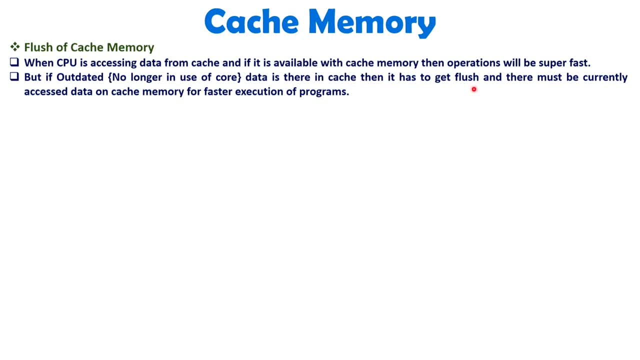 to remove that data means you will have to flush it right. And if you flush that data with respect to operating system, in that case you can say your execution will be fast. But if you know those data are there with cache memory, then program execution will be slower, right So to make. 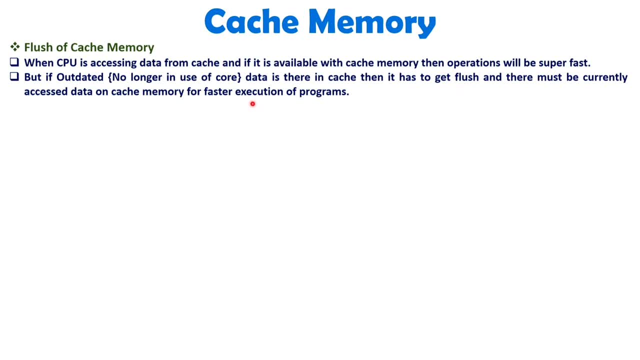 execution fast operating system will flush outdated data right Here, my dear students, operating system updates. currently accessed file into cache memory for faster execution of programs. Here, in order to execute program fast, operating system will remove outdated data from the cache.